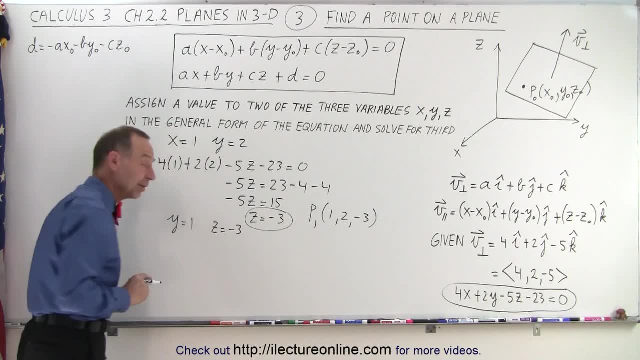 z equals negative 3.. Let's try that. Okay, let's see what that comes out to. So again, we plug that into the equation. So we get 4x plus 2 times y, that 2 times 1,. 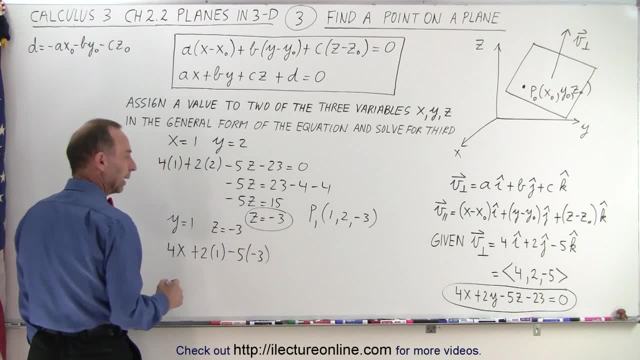 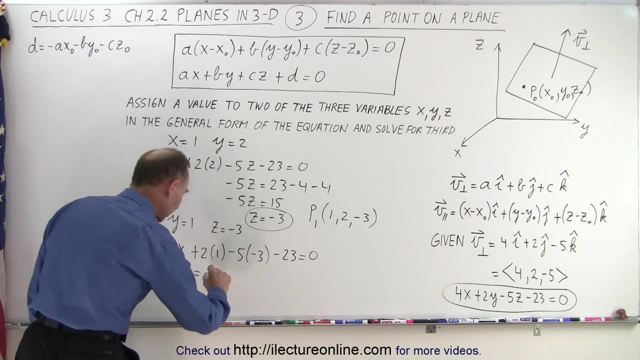 minus 5 times a minus 3, minus 23 is equal to 0.. So here we get: 4x is equal to bring the 23 across, we get 23, minus 2.. And minus times a minus that's plus. that would be minus 15.. 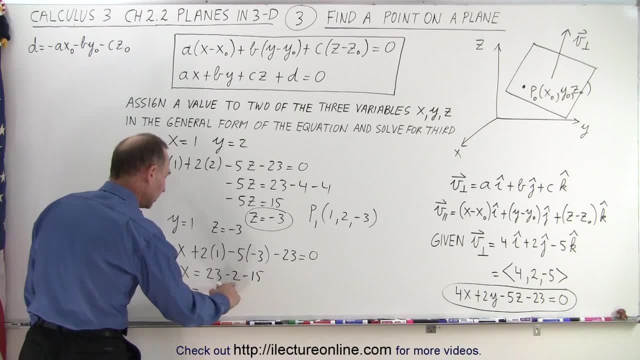 And so we get: 4x is equal to 23,. minus 2,, that's 21,. minus 15, that would be, I think, 4, right, That's 17,, no 6.. So let's see, that would be equal to 6.. Let's try that again. So 23,. 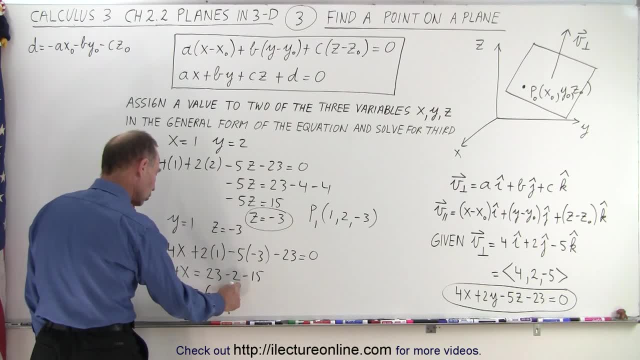 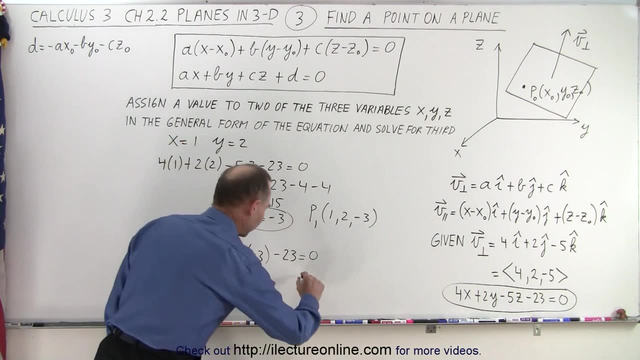 and that would be minus 15, that's 8, minus 2, that's 6.. So we get: x equals 1.5.. All right, and that means that our second point that we found has coordinates 1.5.. 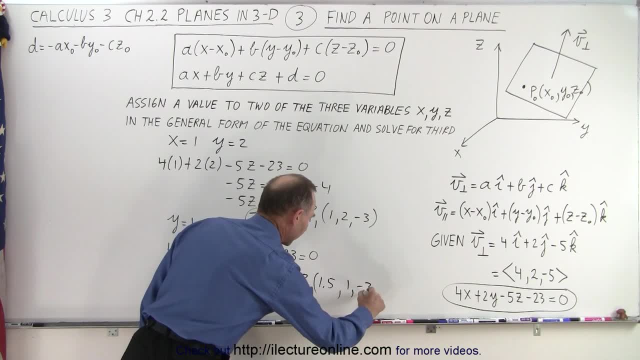 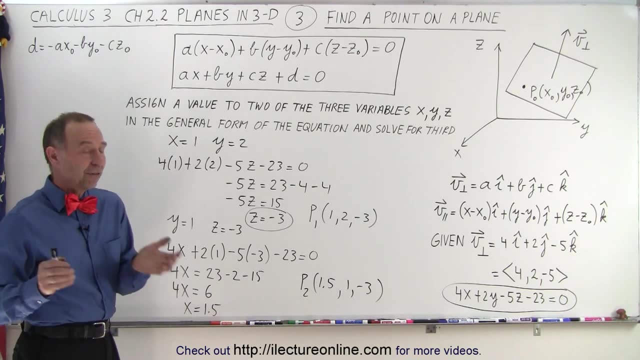 And then we picked 1 and negative 3. There we go, And that's how we find any number of points on the plane. Of course, to find a specific point, that's a different story, because that we don't know, We don't. 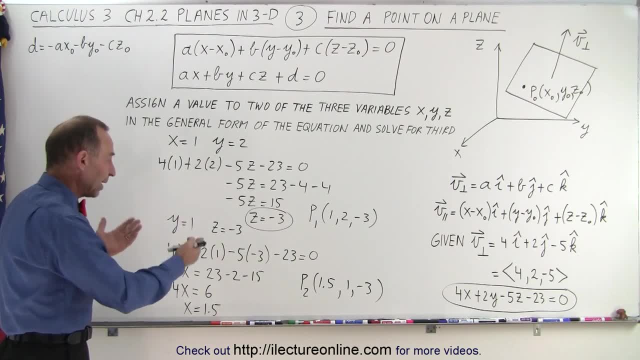 know what x, y and z are, but if you plug in any two values for x, y and z, you can calculate the third using the general formula of the equation, And so you can always pick a point on the plane.